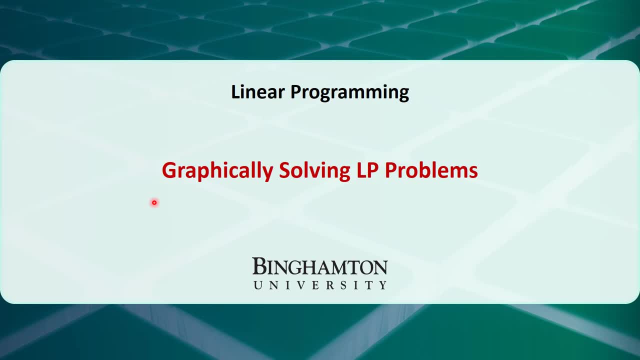 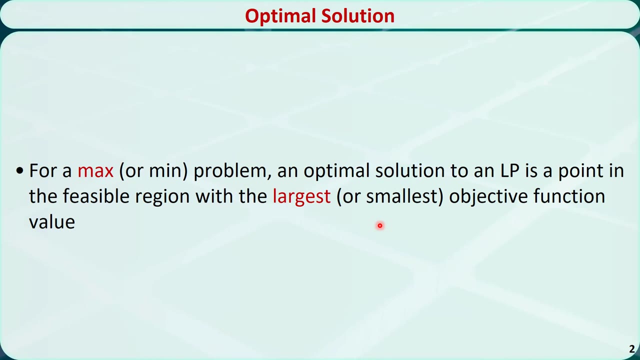 In this video I will talk about how to solve the linear programming problems with two variables using the graphic method. For a maximization problem, an optimal solution is a point in the feasible region with the largest objective function value. If it's a minimization problem, an optimal solution is a point in the feasible region. 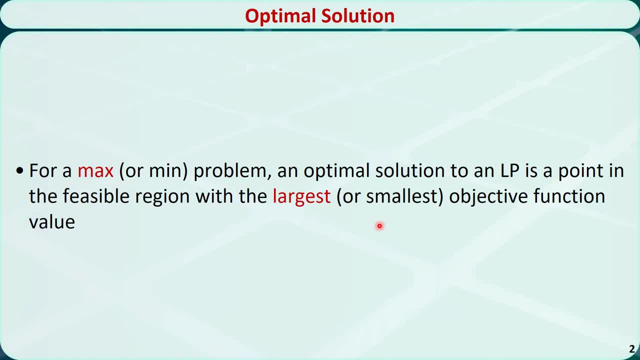 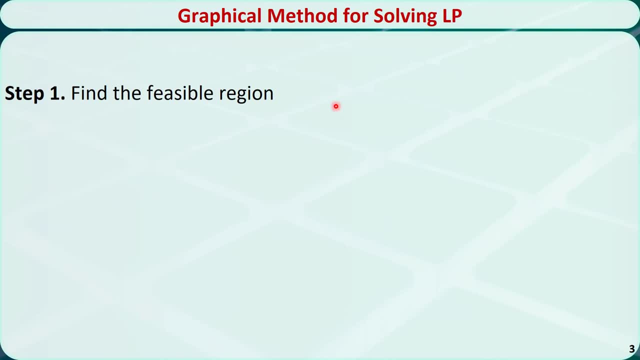 with the smallest objective function value For a linear programming problem with two variables, we can solve it graphically by following these steps: Step 1, find the feasible region. I already introduced how to do that in a previous video. Step 2, find the slope s of the objective function. 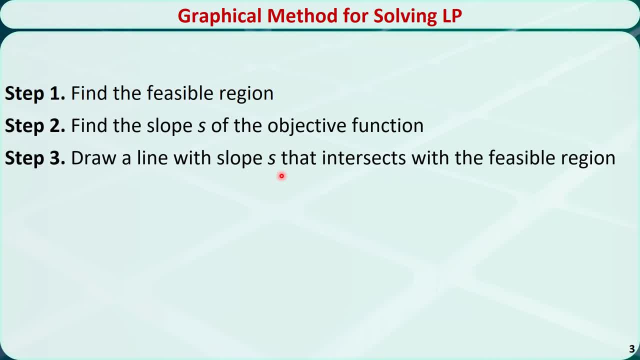 Step 3, draw a line with slope s that intersects with the feasible region. Step 4, move the line in parallel towards the direction that increases the objective function for a maximization problem. If it is a minimization problem, we need to move the line towards the direction that decreases. 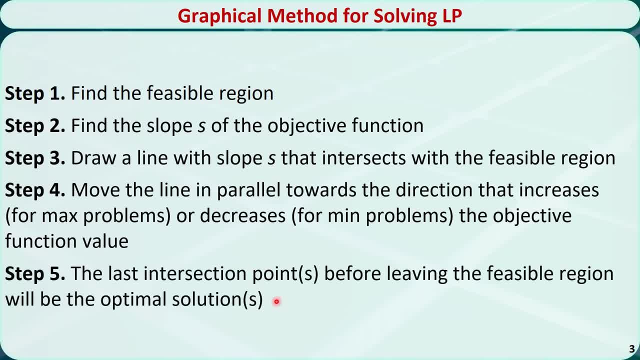 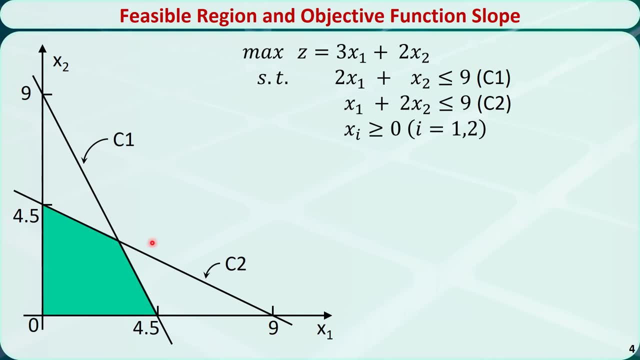 the objective function, Step 5, the last intersection point, a point before leaving. the feasible region will be the optimal solution or solutions. For example, this is a maximization problem with two variables. The feasible region is a point, It is a shaded area. 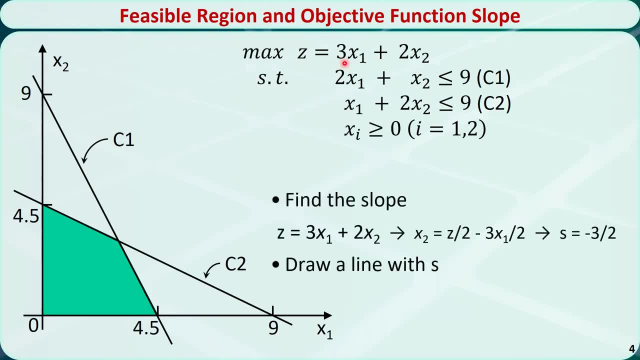 To find the slope of the objective function, we rewrite it: and x2 is equal to z over 2, minus 3x1 over 2, so the slope is negative: 3 over 2.. We draw any line that has a slope s and intersects with the feasible region. 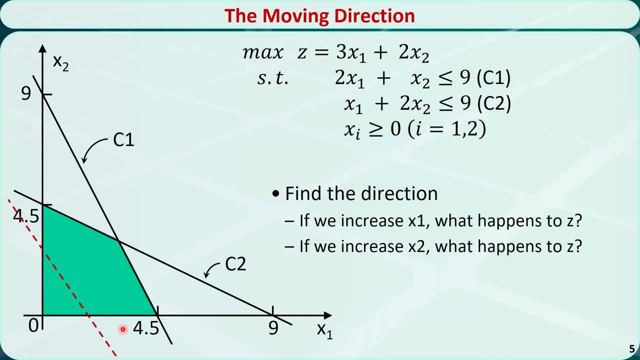 Now let's find which direction to move the line. If we increase x1,, what happens to z? It will increase. If we increase x2, what happens to z? It will increase. So in general, we should move towards the top right corner. 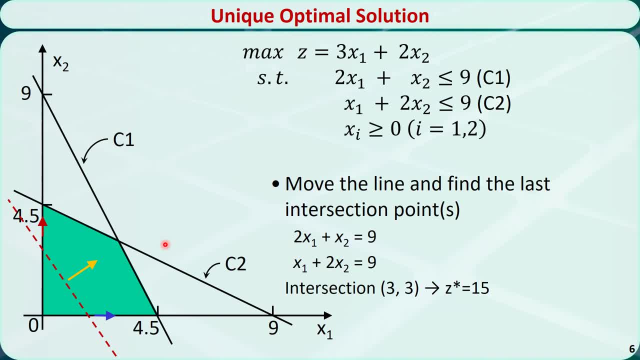 Now let's move this line in parallel towards the top right corner And we find that the last intersection before we leave the feasible region is this point. After this point, the line will no longer intersect with the feasible region. It is the intersection of two constraints. 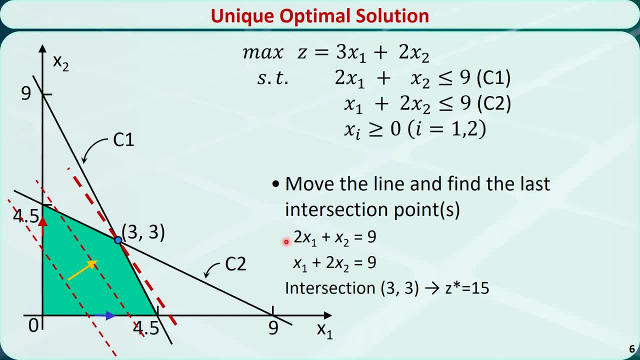 2x1 plus x2 is equal to 2x2.. 2x1 plus 2x2 is equal to 2x2.. 2x1 plus 2x2 is equal to 3x2.. The point is: 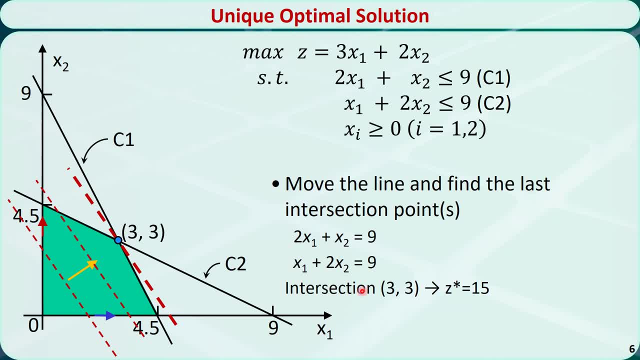 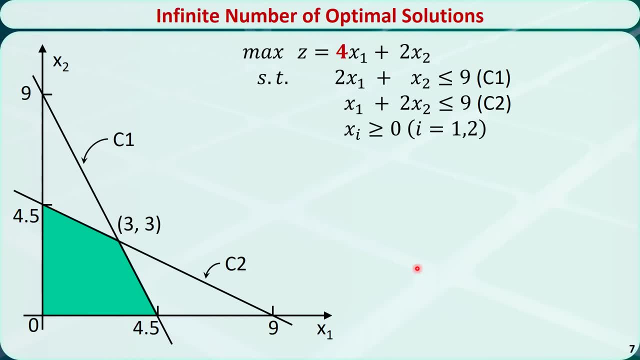 Let's plug these values into the objective function. z star is equal to 15.. This is the unique optimal solution to this problem. If we modify the objective function and change this coefficient from 3 to 4, then we can find in this figure that the feasible region will not change. 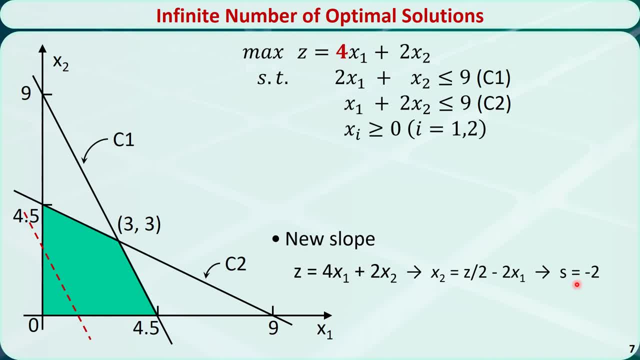 But the slope will be changed from minus 4 to 4.. minus 3 over 2 to minus 2.. It is the same as the slope of the first constraint, c1.. Now let's move this line in parallel toward the top right corner and we find that the 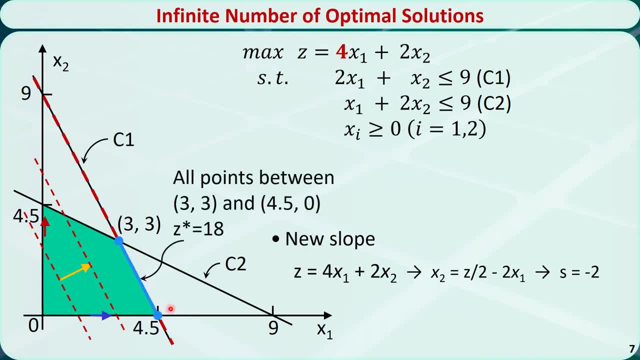 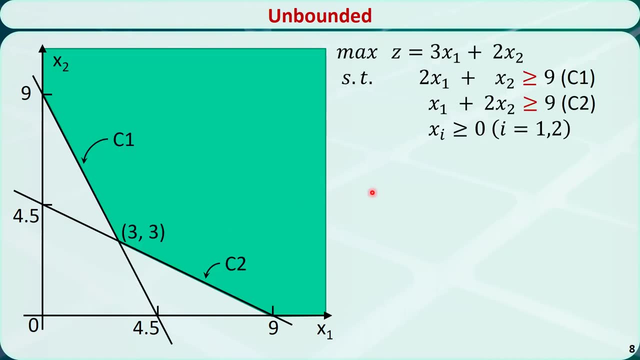 last intersection before we leave the feasible region is this line segment where we have an infinite number of optimal solutions between 0.33 and 0.450.. This star is equal to 18.. In this example, the constraints are changed so they both have a greater than or equal. 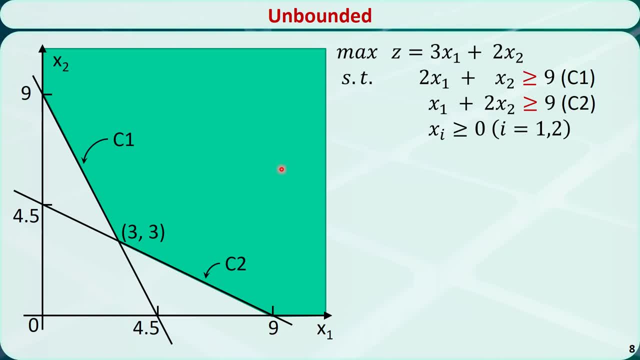 to sign. So the feasible region is changed to this unbounded area. Now let's move this line in parallel toward the top right corner and we find. no matter how far we move the line, we will always intersect. That means the z-value can be arbitrarily large, so the problem is unbounded. 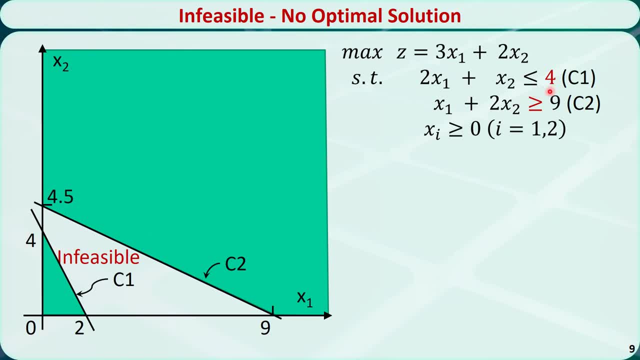 In this example the first constraint is still less than or equal to 2, but the right-hand side is changed to 4.. The second constraint is greater than or equal to 2 constraint. So the feasible region of the first constraint, c1, is below this line and the feasible region 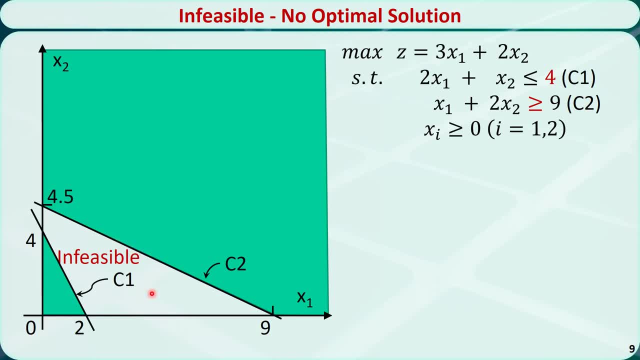 of the second constraint, c2, is above this line. Now there is no intersection between the first constraint and the second constraint. Now let's move this line in parallel toward the top right corner and we find. no matter how far we move the line, we always intersect. 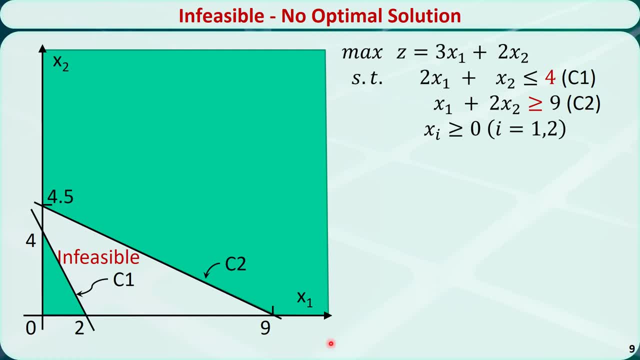 That means the z-value can be arbitrarily large, so the problem is unbounded. The first constraint, c1, has no intersection and the feasible region of the problem is an empty set. So the problem is infeasible. That means there is no optimal solution. 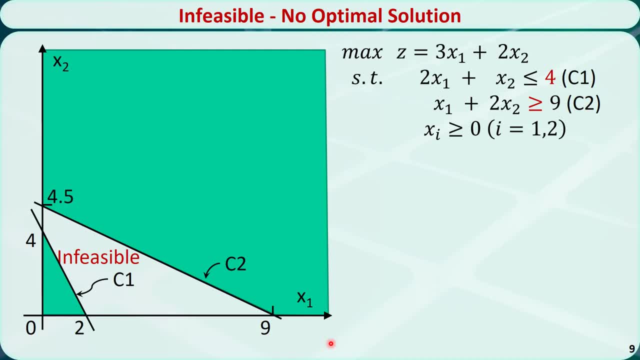 That's how to solve different cases of linear programming problems using the graphic method. Thanks for watching.